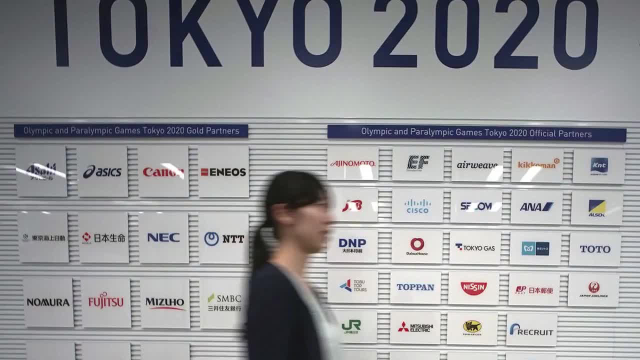 The project was initiated by local politicians In an area long alienated politically and economically in South Korea's rise to prosperity. Some feared people would confuse the city's name with Pyongyang, the North Korean capital. They couldn't count on the automatic support of the huge family-run conglomerates known as Chibol, such as Samsung, Hyundai and LG. When such mega-events were the nation-state's key project, the Chibol were called on and were expected to become the leading participants. 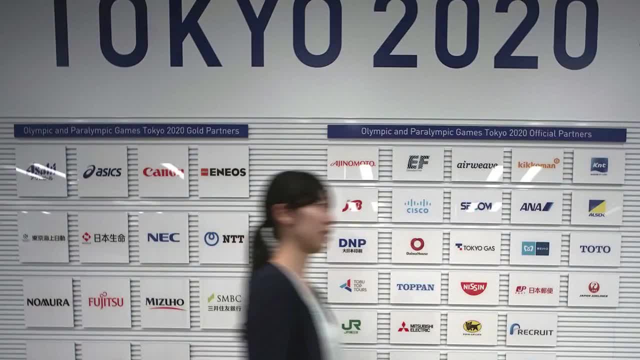 said Ji Yoo-min, a professor at the National University of Singapore who co-authored a book on South Korea's use of mega-events. In the end the national government brought the conglomerates in, first in the bid process and then for sponsorship. That underscores both the outsized role they play in the economy and their close ties with government. They owe a debt to special treatment from the government, which in turn used them to industrialize the country after the devastating 1990 Games. After Pyongchang's bid was rejected a second time, the government called on Samsung and others to help. The president even pardoned Lee Kun-hee, the patriarch of the Samsung founding family, who had been an IOC member but voluntarily suspended his membership after being indicted for tax evasion. The IOC reinstated Lee in 2010 with a reprimand and some restrictions, allowing him to lobby heavily for what became Pyongchang's work. 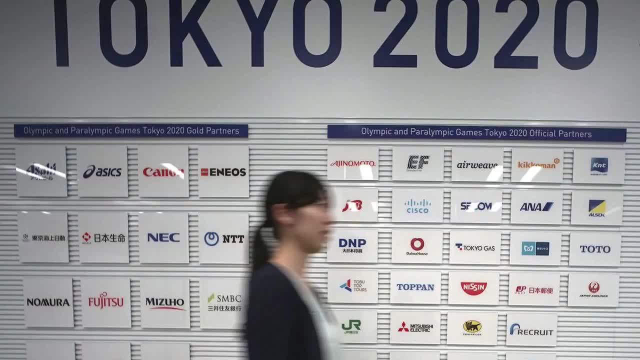 The IOC's winning bid in 2011.. It took three years for the organizing committee to sign its first domestic sponsor, KT Corporation, the country's second-largest mobile carrier. Again, the national government asked the conglomerates for help. All the major ones signed on after the office of then-President Park Joon-hye made a special request and multi-channel pressures for financial assistance. Joo said 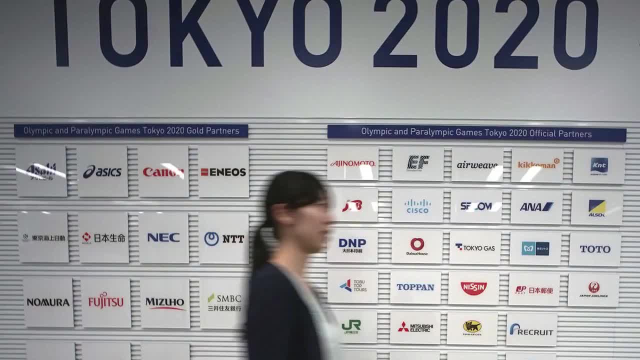 Elsewhere, companies may weigh sponsorship decisions Based more on the marketing benefits. In South Korea, companies make donations out of a sense of duty that they are being part of the national event, said Park Dong-min, the executive director overseeing membership at the Korea Chamber of Commerce and Industry. Sponsors who signed up late weren't willing to give as much because there was less time to enjoy the marketing benefits. A bank that signed on less than a year before the Games significantly reduced its sponsorship. 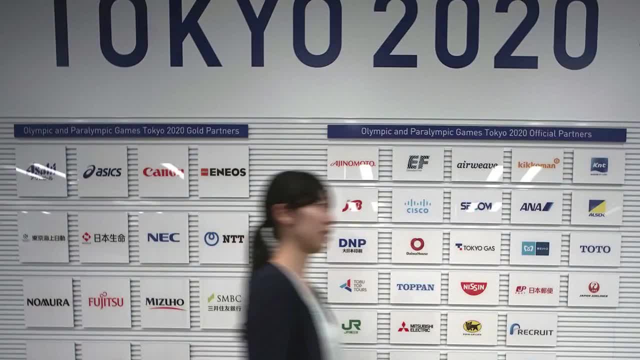 To top it off, a massive sports-related political corruption scandal rocked South Korea in 2016,. just when Pyongchang was making last-ditch efforts to raise sponsorship, Companies showed some reluctance to sponsor the Olympics, said Hyun Chan-wang, director of the Pyongchang Organizing Committee marketing team. Nevertheless, they still joined. The scandal brought down Park the president. 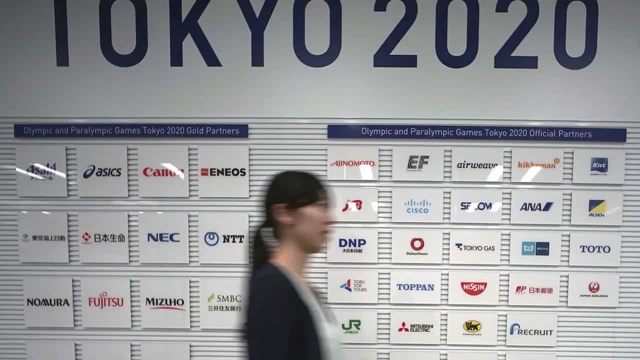 Lee Jae-yong, the heir to the Samsung Group. Lee Jae-yong, the heir to the Samsung Group, received a five-year sentence for bribery. Lee, who has appealed, had become de facto chief of the Samsung Group after his father, Lee Kun-hee, the IOC member, pardoned in late 2009,, fell ill. It was the younger Lee who signed an agreement with IOC president Thomas Bach to extend Samsung Electronics' sponsorship of the Olympics globally through 2020.. Samsung declined interviews for this story With the scandal still fresh in people's minds, Lee said: 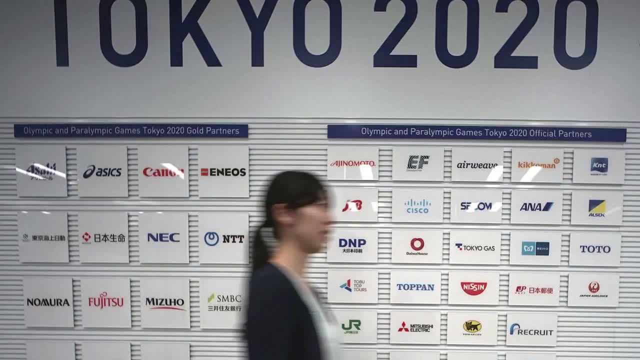 In the minds of the public. major companies have held back from launching full-fledged marketing to promote the Games. Samsung, traditionally, has done consumer marketing through the Olympics, but because its chief is in jail, it cannot do as much these days, said Kim Do-kyun, a sports professor at Kanghee University Graduate School of Physical Education. The Pyongchang Games were the biggest victim of the scandal, he said. 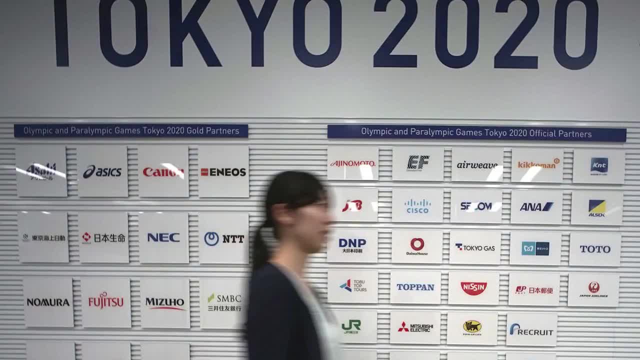 Summer of 64.. The president of Japan's biggest toilet manufacturer was seven years old when the Olympics first came to Japan. Toto Limited made news in 1964 for its prefabricated toilet and bath units that helped speed the construction of a luxury hotel, the new Itani, in time for the Games. The company, now known for high-tech toilets that baffle some foreign visitors, is back as a sponsor of Tokyo 2020.. I feel our company and the Olympics have been bonded by fate. Toto president said. The second-ever president, Madoka Kitamura, said at a sponsorship signing ceremony at the same hotel last year: The $2.7 billion in sponsorship for Tokyo 2020 is more than three times the original estimate. By comparison, sponsorship revenue was $848 million in Rio de Janeiro last year and about $1.2 billion for both London 2012 and Beijing 2008.. The Winter Olympics typically attract less, though Russia raised $1.2 billion in 2014.. Analysts attribute Tokyo's success to both patriotism and a sense of nostalgia for the 1964 Summer Games. They were much more than a sports contest. 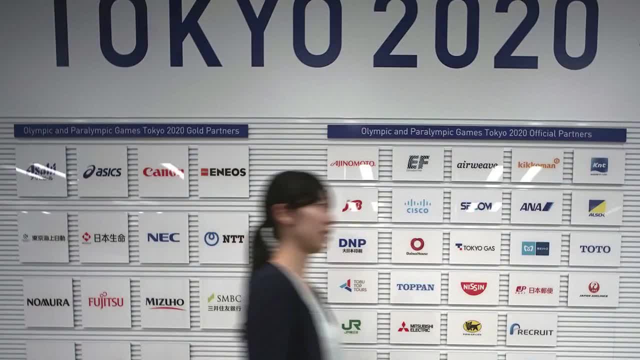 for Japan, They were a moment of pride, marking the country's return as an industrial power after the devastation of World War II and a seven-year US occupation. All of Japan still recognizes the unique role that the 1964 Olympics played in Japan's stepping out onto the world stage. 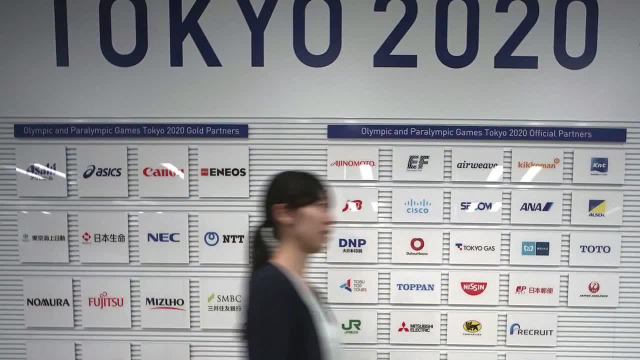 said Michael Payne, a former IOC marketing director who now works as a consultant, Many of the CEOs of top Japanese companies would have been young kids back in 64, and are very aware of the role those games played for the psychological recovery from the Second.